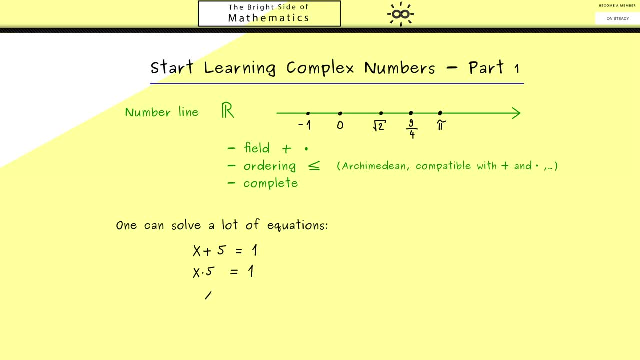 we have a field. Then another equation we solved is: x squared is equal to 2.. This one leads to the square root of 2, which is in r by completeness. However, this does not mean that we are able to solve any quadratic equation. For example, the quadratic equation x squared is equal to minus 1. 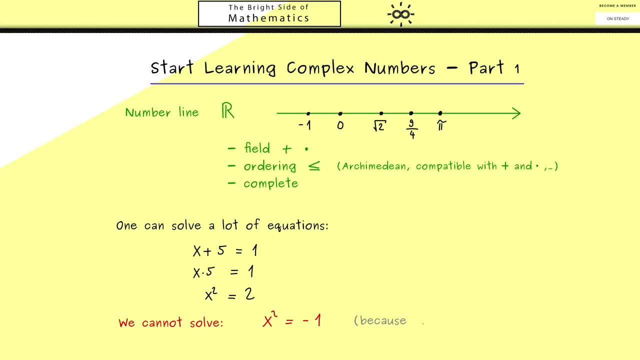 has no solutions. This is not hard to see, because you can show that any square in the real numbers is greater or equal than zero. And we also need that minus 1 is less than zero. Here I can tell you, if you just work with the axioms of the real numbers, it's a good exercise to show both of. 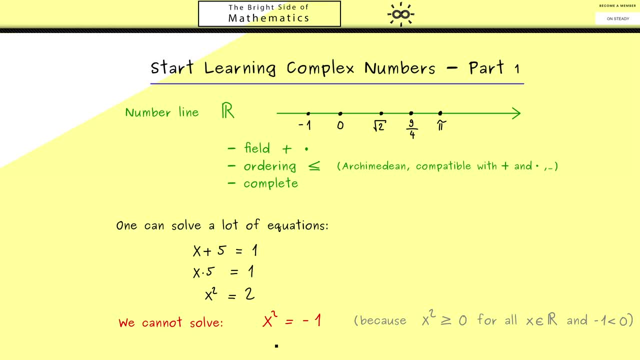 these things, Then this implies that this simple equation does not have any solution. However, for us it makes sense that we extend our numbers such that this equation has solutions. The first thing you should note here is that x squared is nothing else than x times x. I say that because the same equation with the addition. 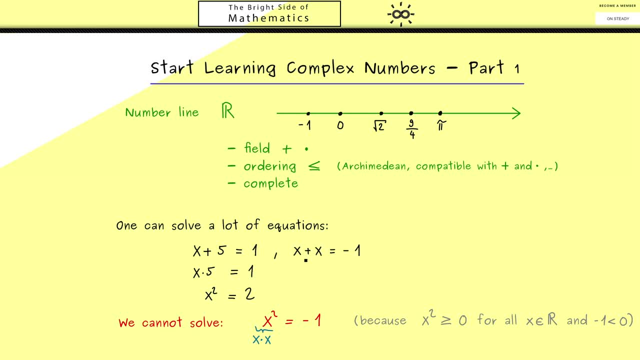 is solvable. So surprisingly, the addition and the multiplication act differently in r, which also has something to do with the ordering. Hence our idea is to expand the number set such that we can solve such equations here. but we already know that we can't conserve all the properties in r In order. 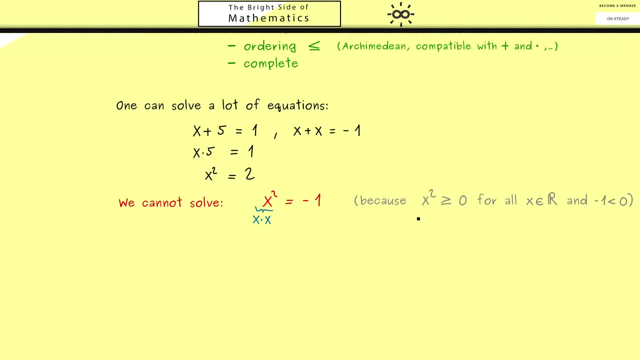 to see what we can do, let's look at the number line again. First, let's fill in the number 0,, 2 and 4.. Now you know, we can go from 2 to 4 just by using multiplication. we simply multiply by 2.. 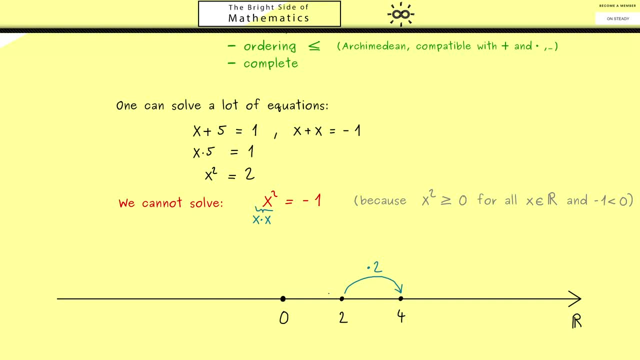 However, the interesting thing is now that we can split this big jump into small jumps. We just multiply by a number that is a little bit bigger than 1.. You see, the smaller the one jump is, the more jumps we need. Ok, this splitting up does not work when we want to jump to minus 2.. 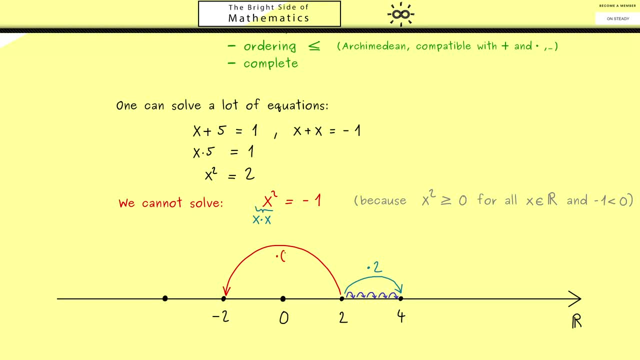 For this big jump we have to multiply by minus 1.. Also interesting here: if we multiply again by minus 1, we get back to 2.. So here you see: multiplying with a negative number is different than multiplying with a positive number. 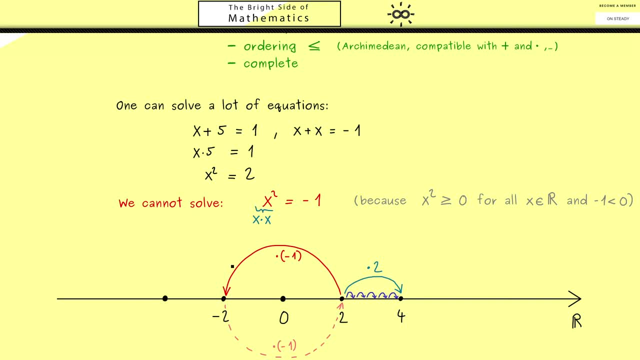 Because in the first case we immediately change the side of the number line. Now, looking back to the splitting of the jump for positive numbers, here we can see the equation from above, Because doing two jumps with the number x means we have x squared is equal to 2.. 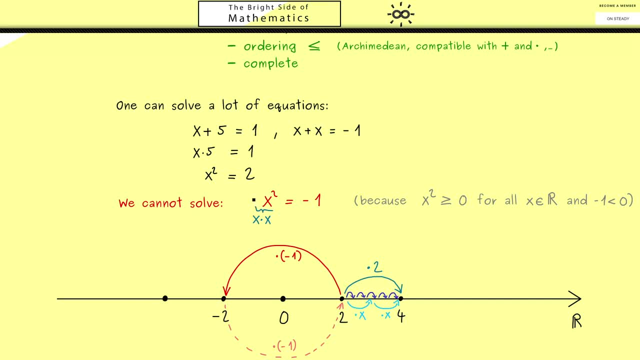 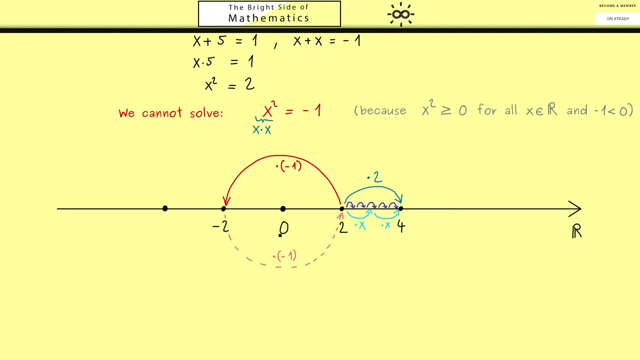 So exactly this equation where we know we have a solution. Now you might see the problem: how can we split up this jump into two parts? Ok, By looking at this picture you might already see we could just add another direction for the numbers. 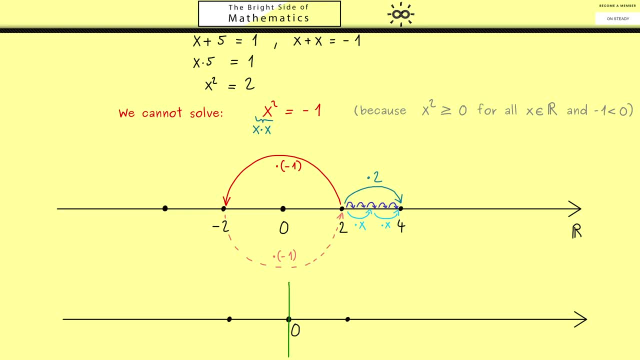 Therefore, the idea is that we also include a y-axis. now Here, jumping from 1 to minus 1 is still given by multiplying with minus 1.. However, now we are able to split it up into smaller parts, For example into two parts where we multiply with the number x. 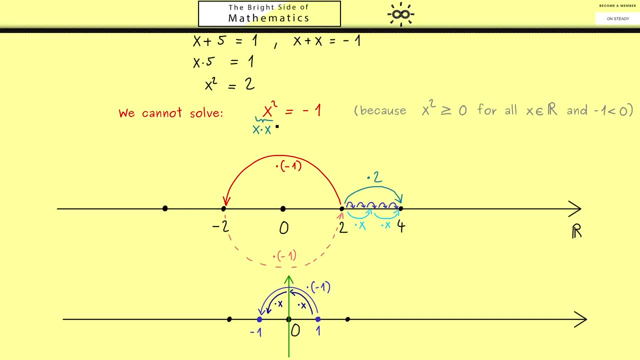 And there you see, this is our equation from before. x squared is equal to minus 1.. Hence you see, the number we search for is this point in the plane. So we need a new name for this number. We call it i. 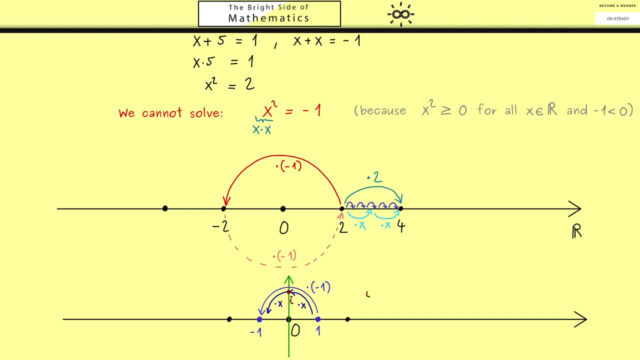 Now, with our picture in mind, this i is now a special number Because when we multiply i with itself, we get out the jump minus 1.. Or to put it in other words, i squared is equal to minus 1.. And this is now the important formula we should remember all the time. 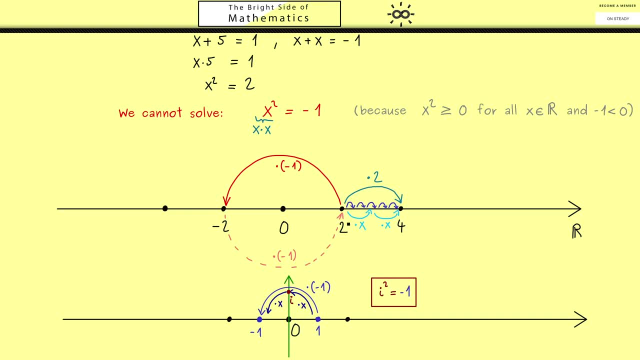 Ok, With all this, we have some idea what our goal is- to expand the number set- And how we can reach that goal. Extending the number line into a second direction is, of course, a completely new idea. Therefore, we really have to do this in a formal way. 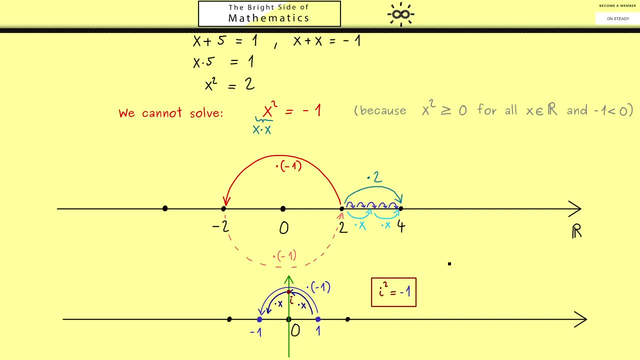 What we can do in the next video In this way. I hope I see you there And have a nice day. Bye.